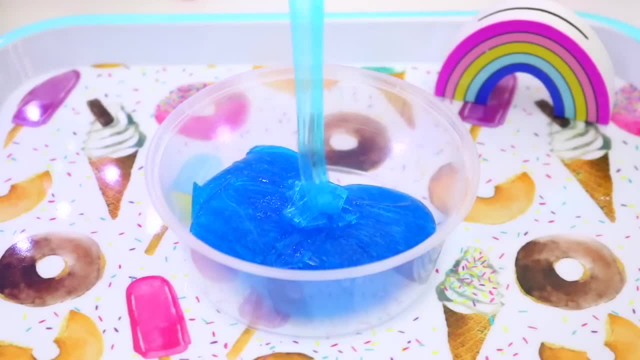 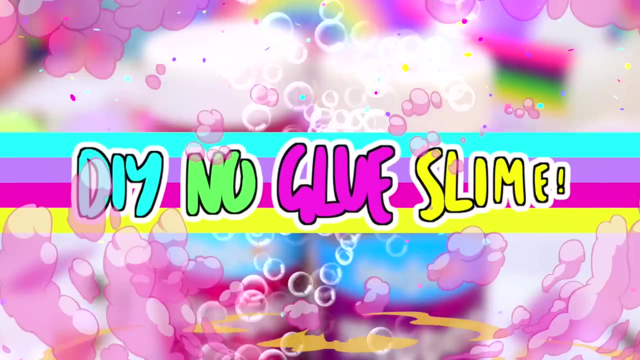 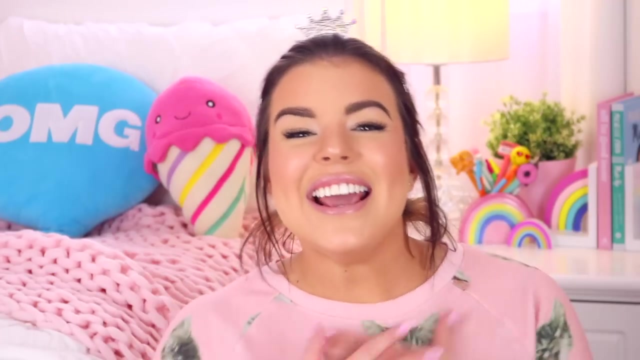 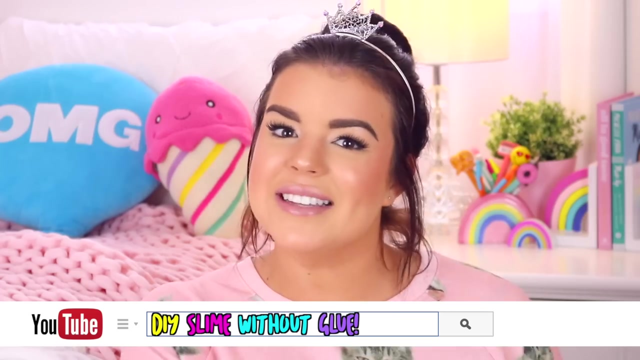 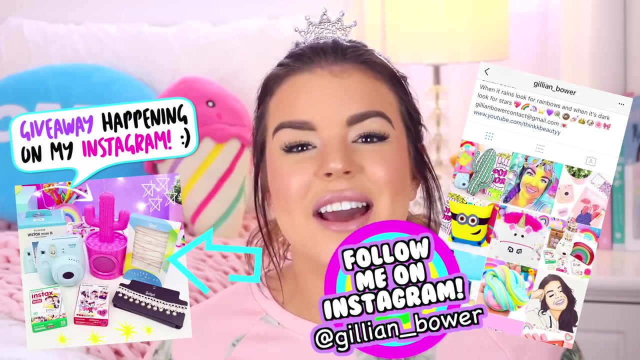 Hey everyone, it's Jillian, and for today's video I thought it would be so much fun to show you guys some more super easy recipes to make slime without glue. So in my last video I showed you guys how you can make a really awesome fluffy slime without glue, and you 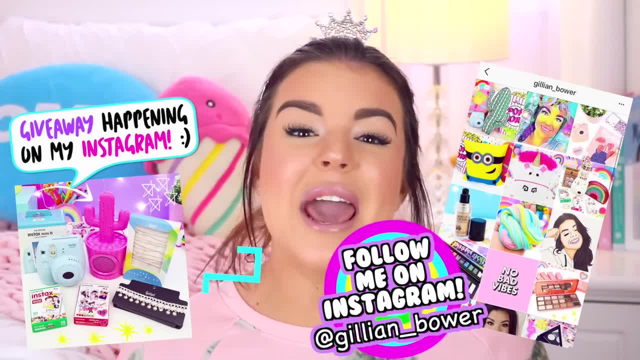 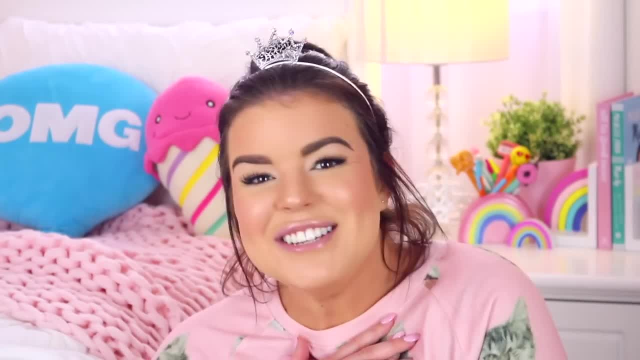 guys seemed to really like that and found it super helpful. So today I'm going to be showing you four more no glue slime recipes. If you guys enjoy watching this video and you love slime just as much as I do, it'd be awesome if you let me know by giving this. 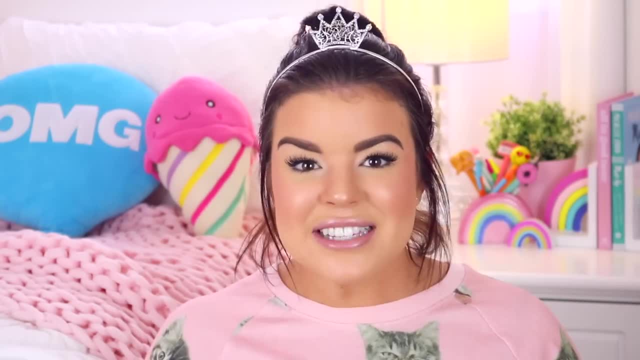 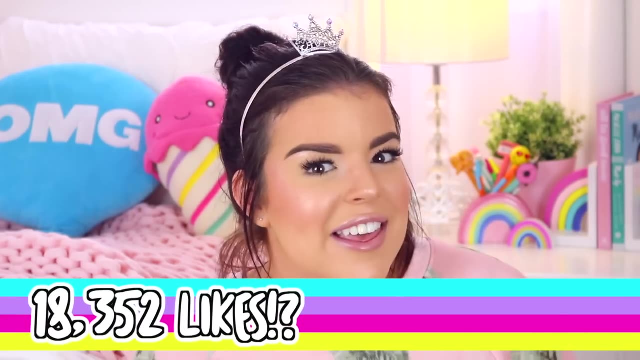 video a big thumbs up, and let's see if we can get this video to 18,352 thumbs up. That would be so awesome and I totally think you guys can do it. Now. if this is my first video that you're seeing, then hello, my name is Jillian and 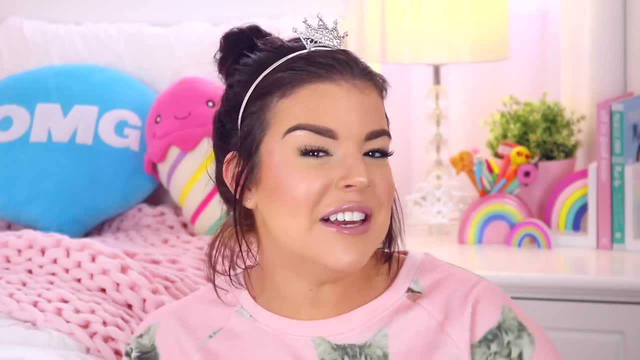 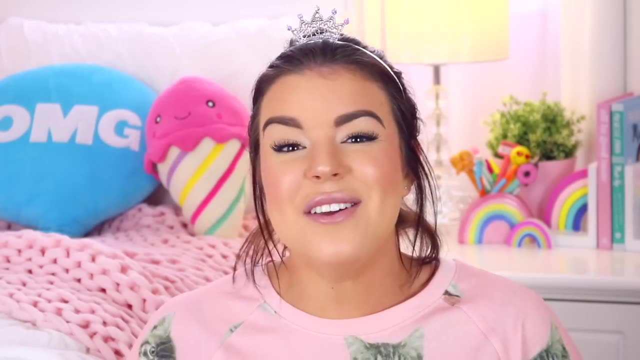 I am so, so happy that you found my channel, and if you'd like to see more videos from me in the future and you haven't already subscribed, then just go ahead and click that subscribe button and then whenever I upload a new video, you'll be able to see it. Now I am super excited. 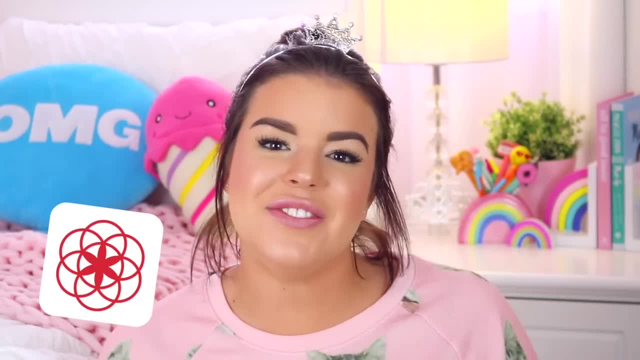 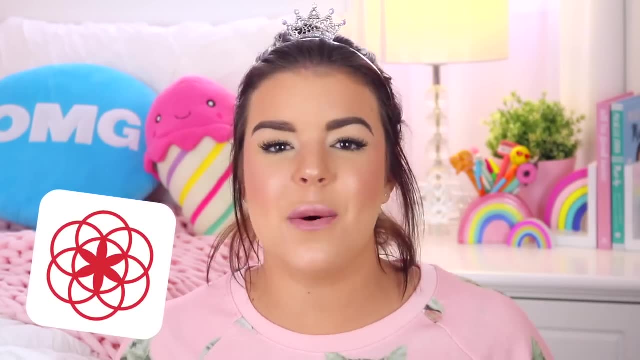 because I have partnered up with the app Clue for today's video, and Clue is basically an app that helps you track your period and figure out everything that is going on with your body. So, honestly, I wish this app had existed when I first started my period, because it would 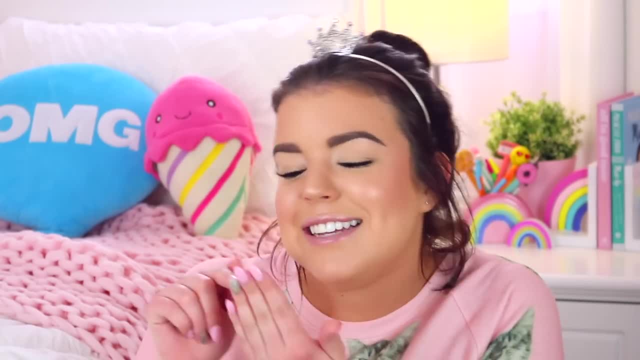 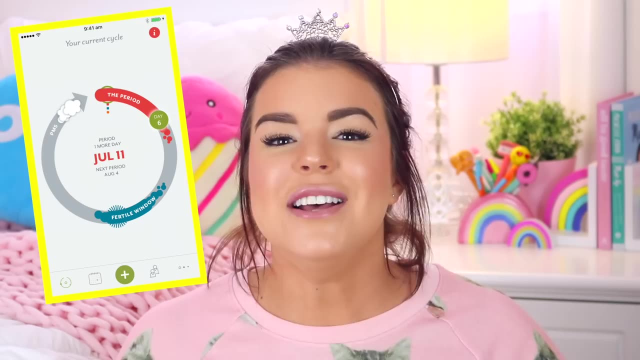 have been so helpful. I remember sitting there like counting the days on the calendar, trying to figure out when my next period was due, and I would always get it wrong and I'd always mess it up. So I am so happy that this app exists and I just have to share it with you. 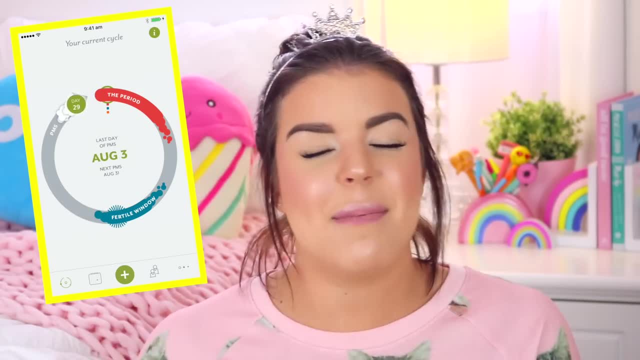 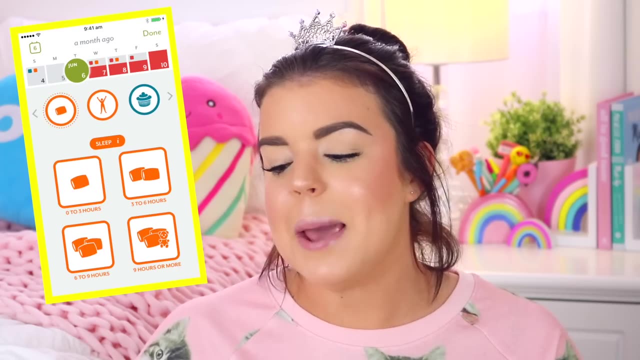 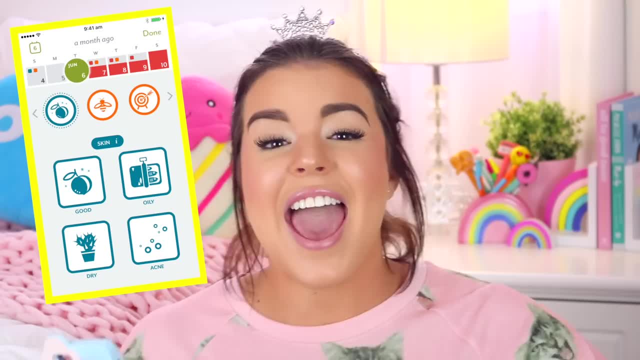 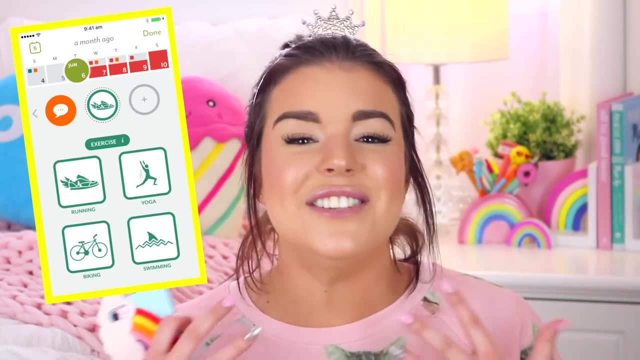 the information that you can add about how you're feeling and what is going on with you today, And then this app will basically just take on that data and it will tell you how you're going to be feeling on certain days and it will tell you what's going on with your body. 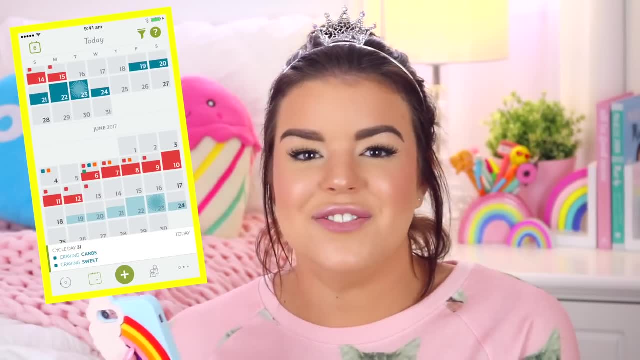 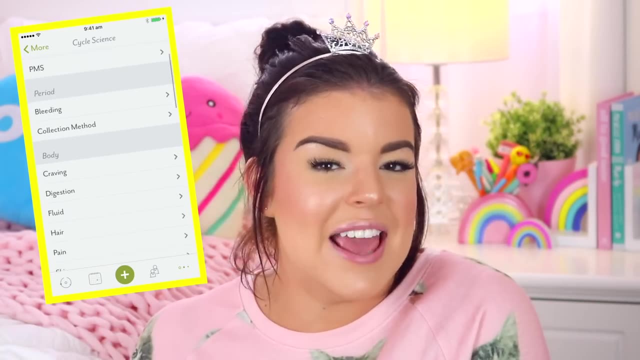 So my favorite part about this app- and I was so happy to see that it had this feature- and I know that so many of you guys are going to find this helpful- So if you click on cyclo signs, it will take you into a list where you can see a bunch. 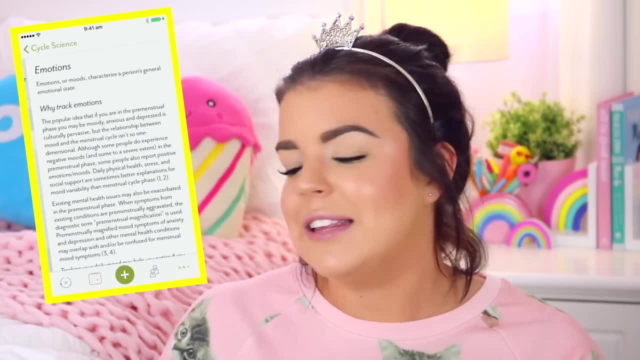 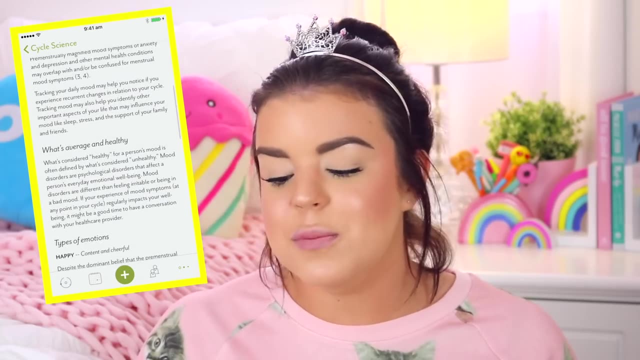 of different feelings, emotions and just everything to do with your period. while clicking on the. click on something- For example, I've clicked on emotions- It'll tell you why it's important to track emotions. It'll tell you what's healthy, what's normal. It'll tell you the different. 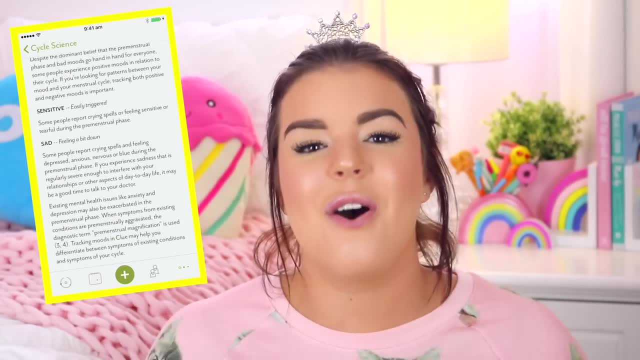 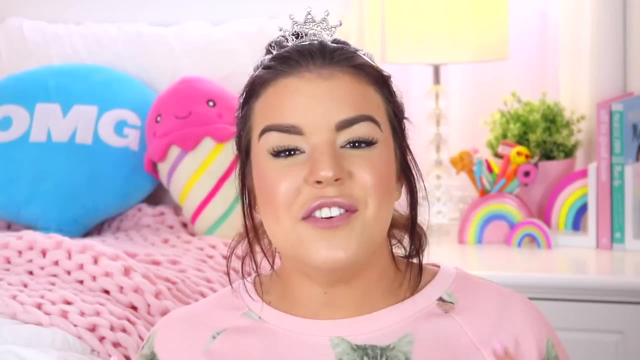 types of emotions. So you'll basically just get to learn a lot about what your body is doing, why it's doing that, and I just love that all the information is in one spot. So if you feel like you need this app in your life- and seriously I am so happy that it- 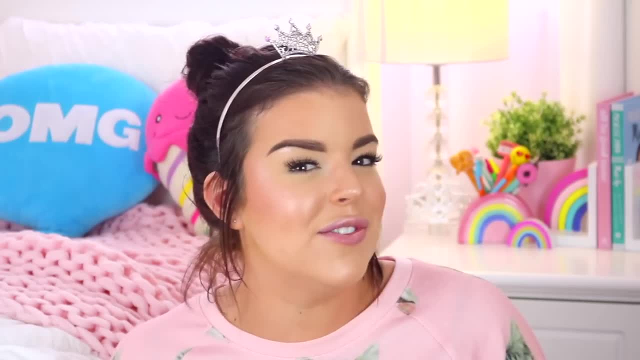 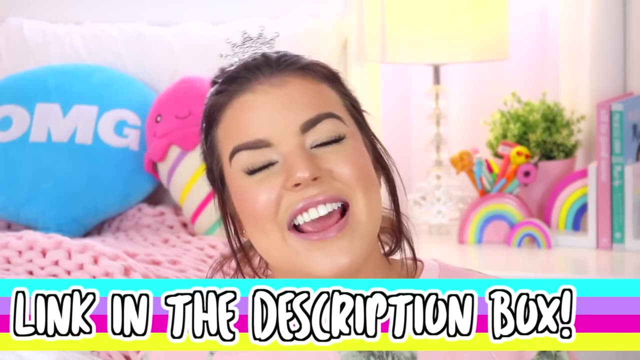 exists and I just really wanted to share it with you guys because I know that a lot of you will find this super helpful. You can download it for free on iOS or Android, and I will leave a link to download it in the description box, so make sure you check that. 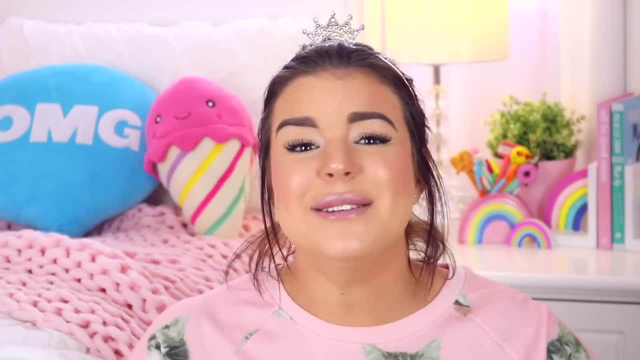 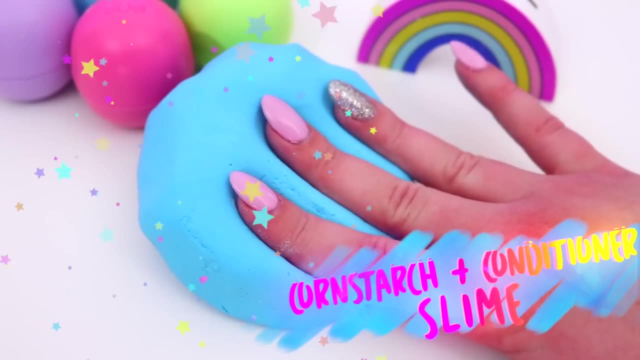 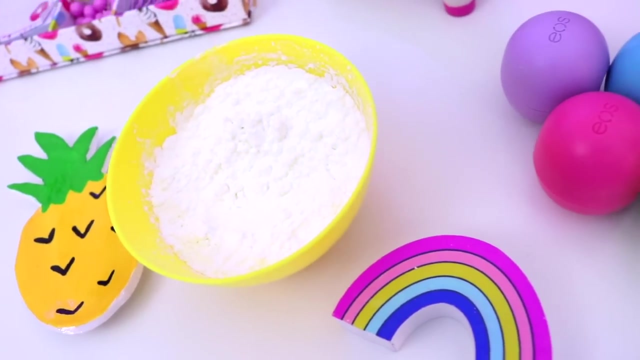 out, So I think it's time that we jump into the video and let's start making some really awesome slime without glue, Starting off with this super simple no-glue slime. and technically, this only uses two ingredients if you don't use food coloring, So the first thing you are going to need is 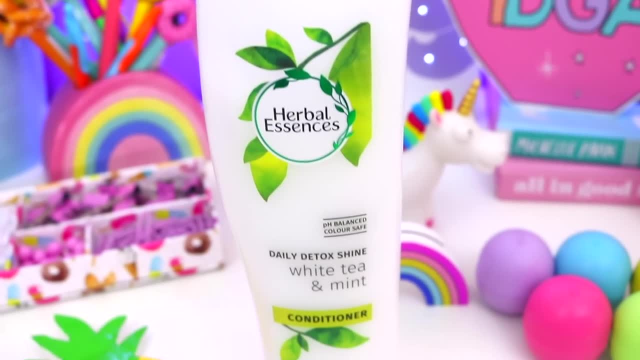 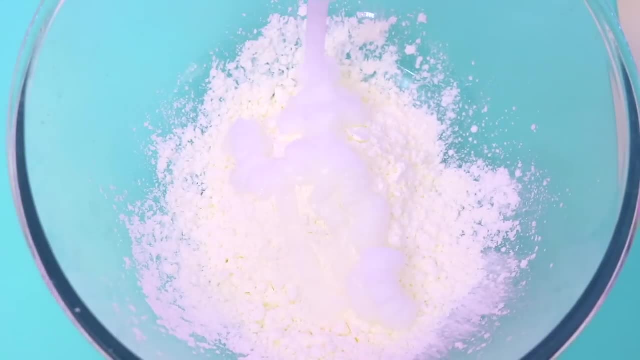 some cornstarch, So just add this to a bowl. and then you're also going to need some hair conditioner, and just add this to the bowl as well. Now I started off adding about equal parts and then mixing it together, and it takes a while to mix in, but just be patient with it and 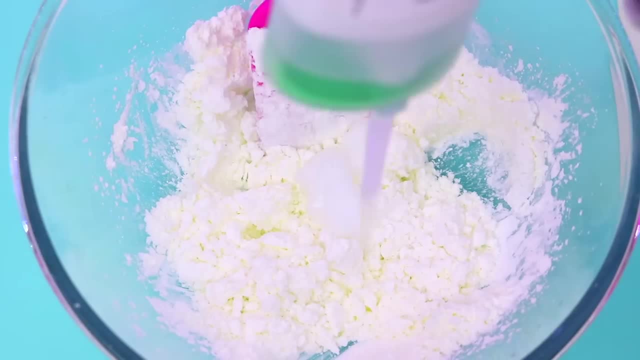 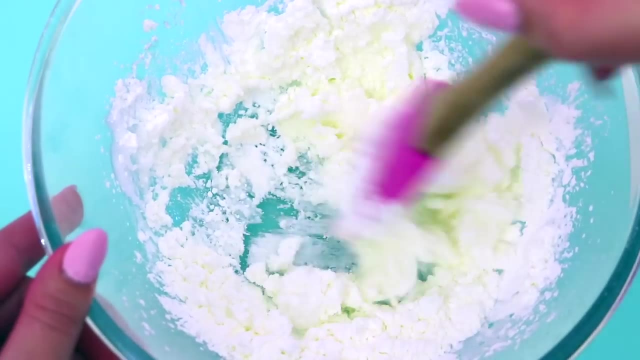 you'll see it start to combine And if your mixture is too wet then add more cornstarch, and if your mixture is too dry, then add more conditioner. But just keep mixing it together until you get this awesome, really soft dough. 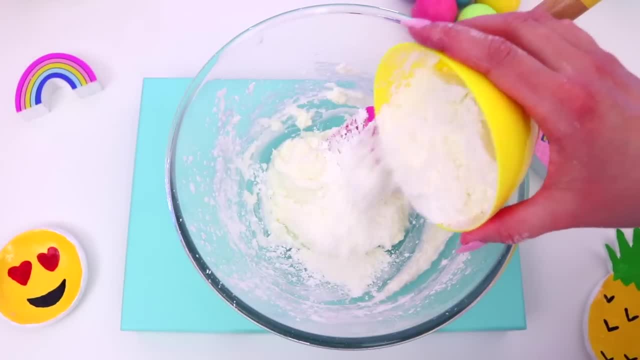 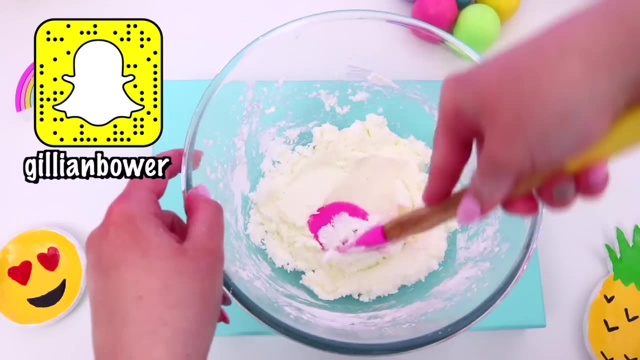 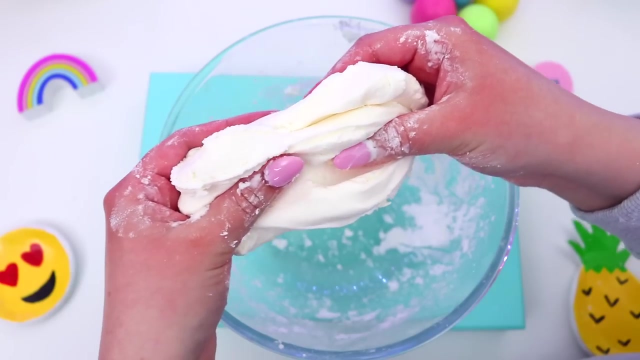 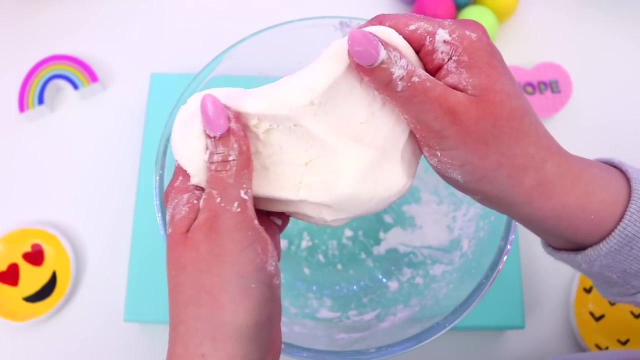 If you don't want to use a spatula, you can also use your hands to mix it together, and this works as well. And then, once it's all mixed together, you should have this super soft and stretchy dough, and this is such an awesome texture. It feels so awesome and 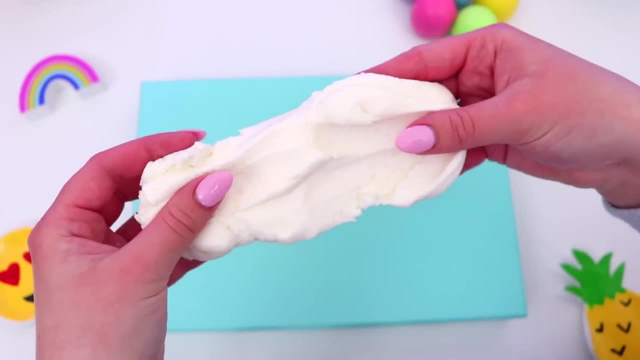 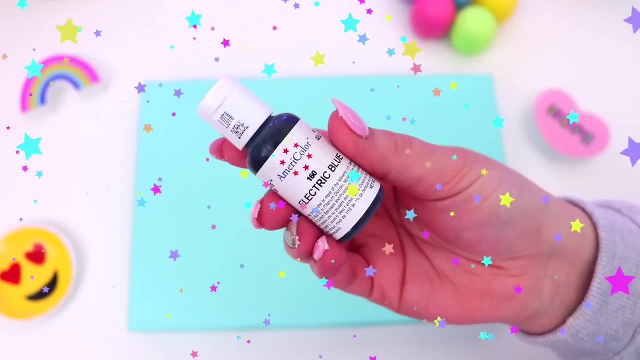 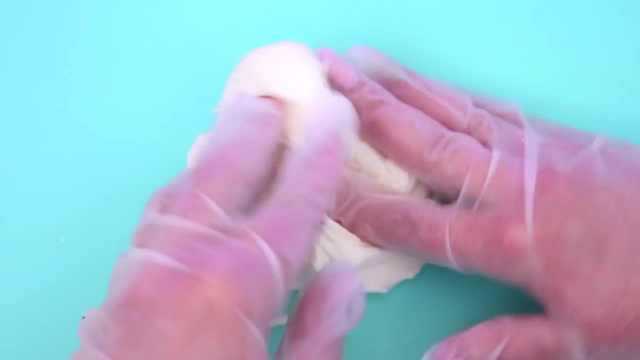 I'm just so excited. Now I'm going to add some food dye to give it an awesome color. and here I'm adding blue food dye and then I just put on some gloves to mix in the food dye because I didn't want. 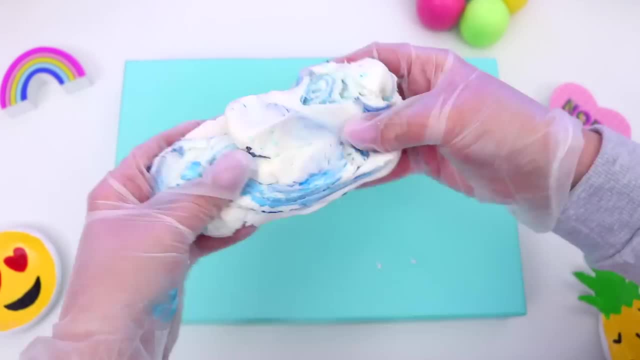 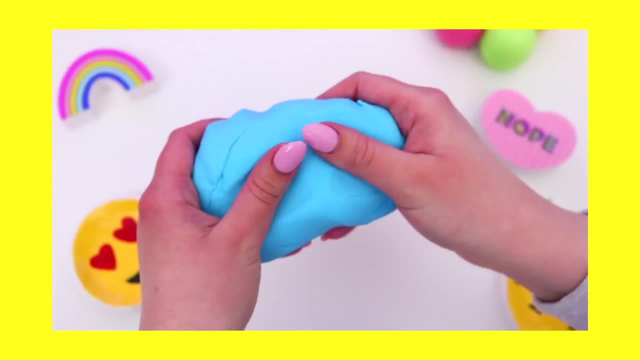 to stain my hands blue. So then just mix the food dye into the cornstarch and conditioner mixture and see it start to change color, and this is so much fun. I love, love, love love this no-glue slime, and I know it's not like the traditional slime texture, but 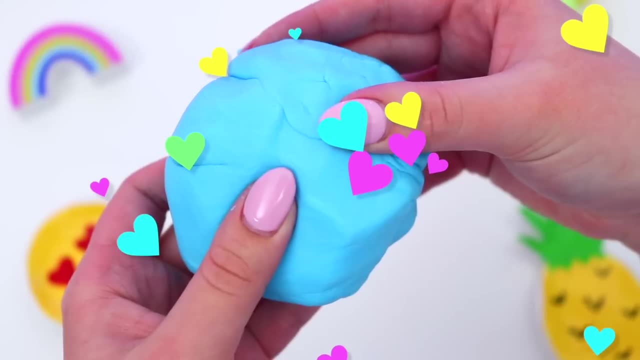 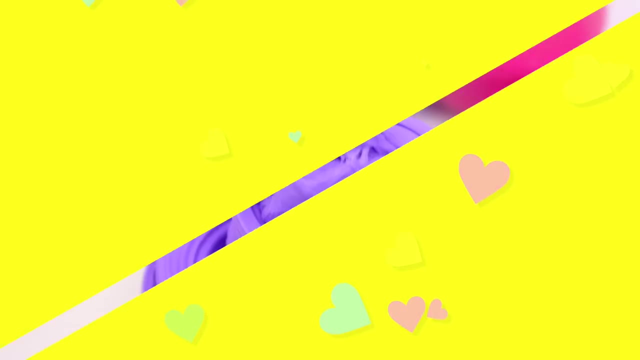 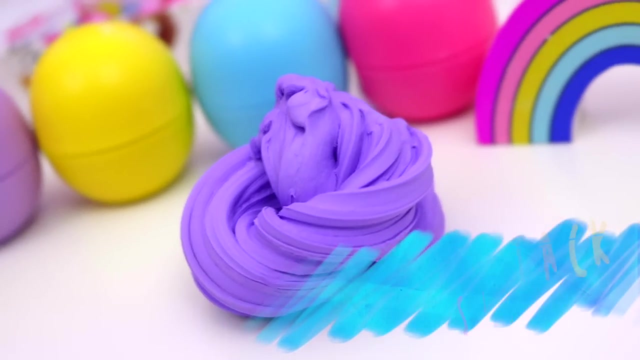 I know a lot of people have cornstarch and conditioner at home, so if you have those ingredients, you can just mix them together and make this super awesome, super easy no-glue slime. So now, moving on to another two-ingredient slime, if you don't count the food dye and 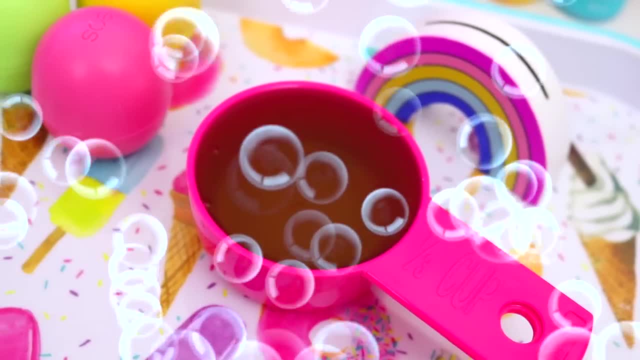 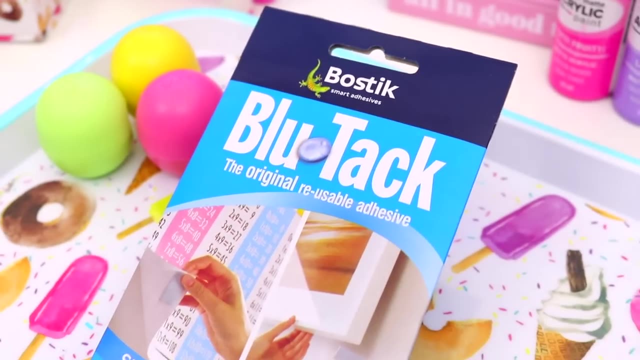 we are going to be making Blu-Tack slime, So the first thing you're going to need is some hand soap. So just add a little bit of this hand soap And then you are, of course, going to need some Blu-Tack. so just take some and start working. 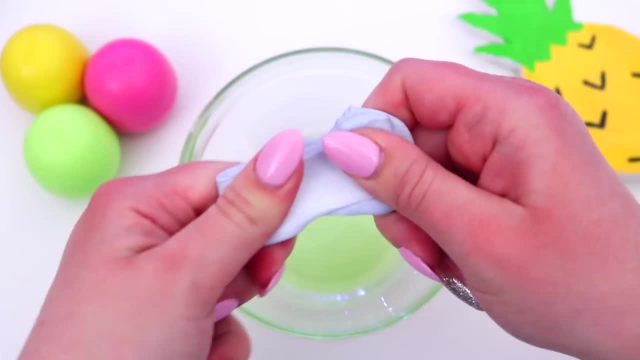 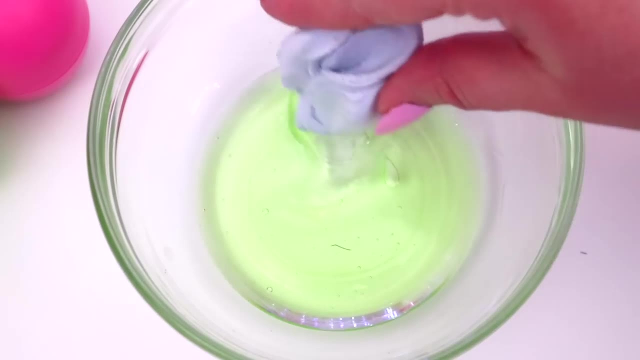 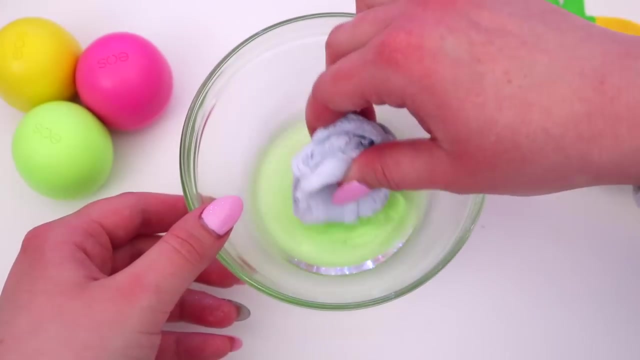 with your hands to warm up the Blu-Tack, to make it a bit stretchier and a bit easier to work with. So then all you need to do is dip the Blu-Tack into a little bit of the hand soap and then start pressing all the Blu-Tack and the hand soap together so the hand soap mixes in with. 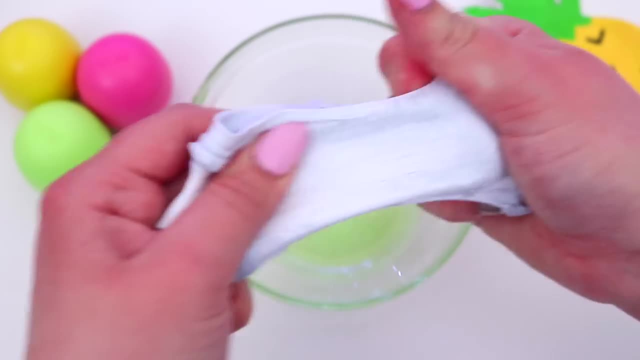 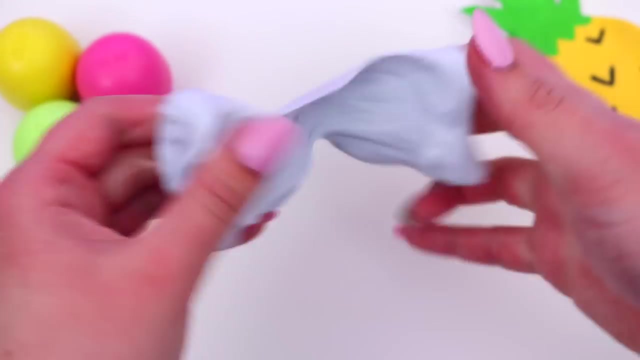 the Blu-Tack And then just keep on repeating this and you will find that the Blu-Tack will get softer and stretchier the more soap you add to it. But I found that if I added too much soap it actually made the Blu-Tack quite sticky. 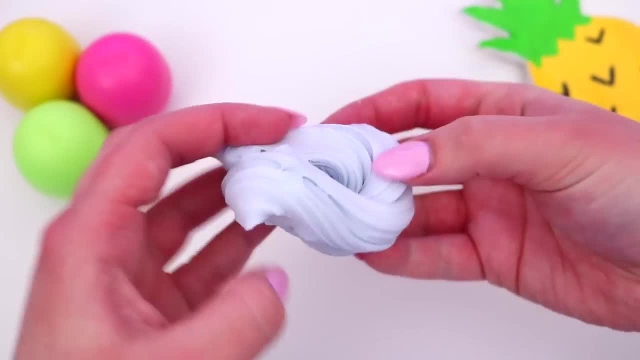 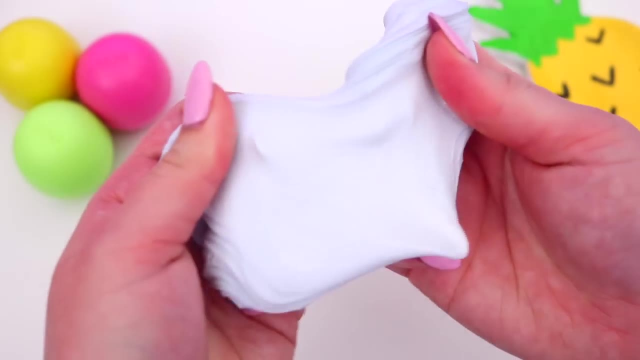 so just keep an eye on that when you are adding the hand soap. So I love, love, love this slime so much. it made the Blu-Tack so light and like really, really soft. It was such a cool texture and it was nothing like regular Blu-Tack and I can't believe. 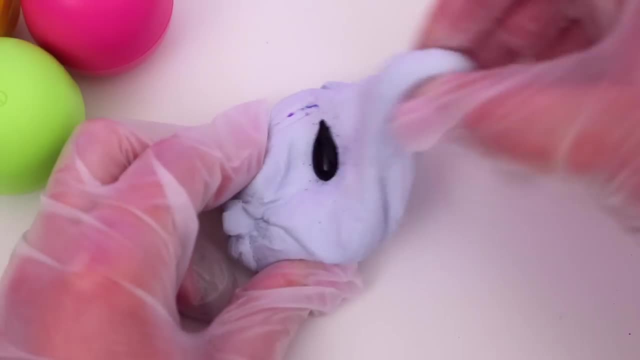 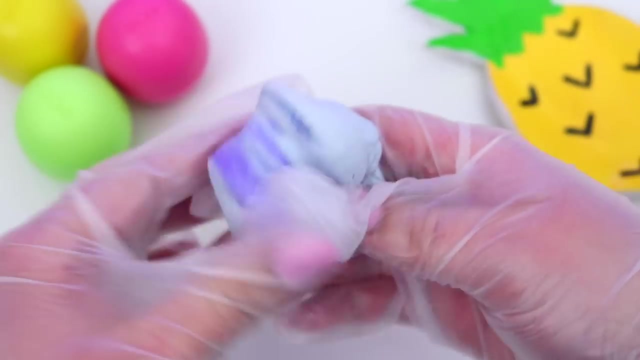 that it changed so much much just with hand soap. So I of course wanted to make my Blu-Tack Slime a really fun colour. so here I added some purple food dye. and then again, wearing gloves, I just mixed the food dye into the Blu-Tack Slime. 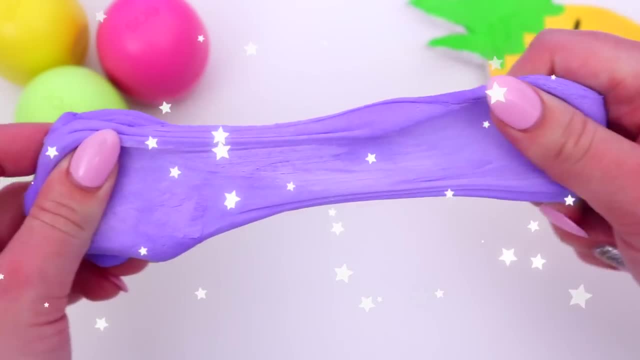 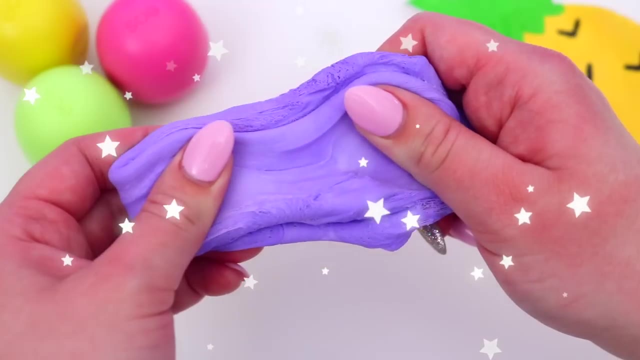 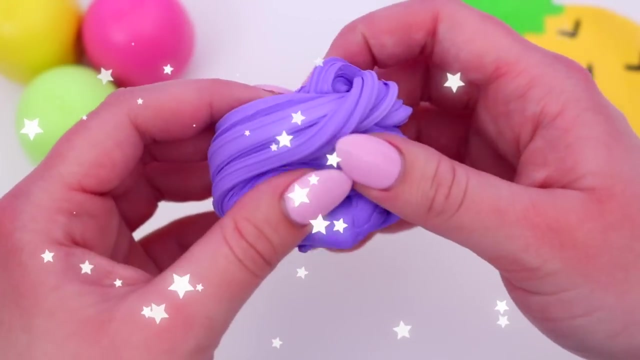 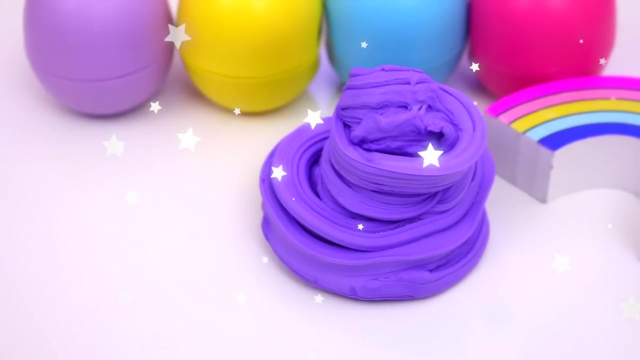 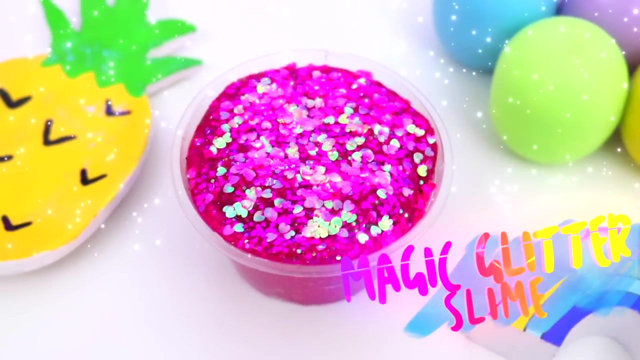 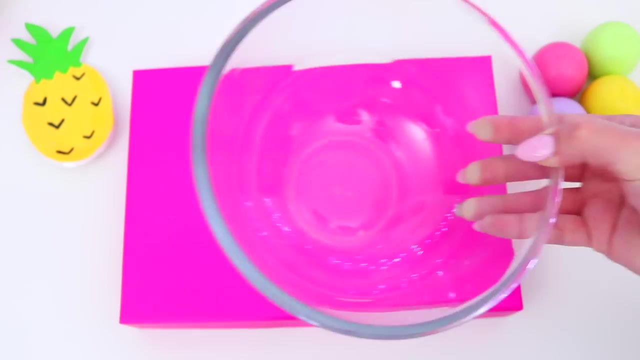 And I love this Blu-Tack Slime so much. It's not like any other texture of slime, but it's still super stretchy and super soft and it was so much fun to play with. So now moving on to this No Glue Glitter Slime, and this is probably one of the prettiest slimes I've ever. 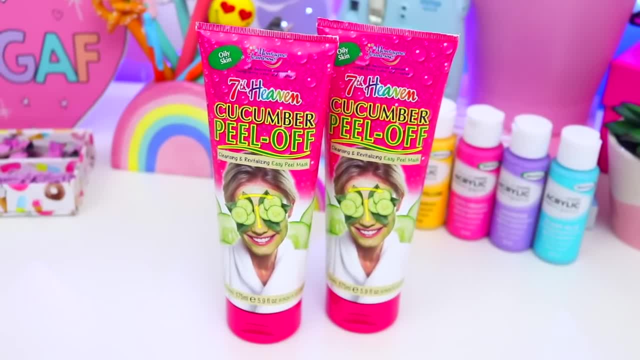 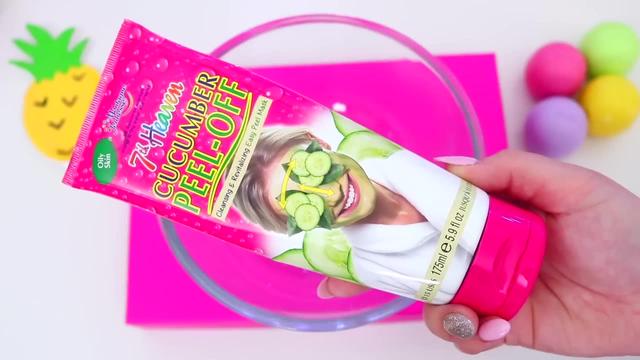 made. The first thing you're going to need is a bowl, and then you're going to need some peel off face mask and you need to check the ingredients on the back to make sure it contains polyvinyl alcohol. So then just take your peel off face mask and add some to a bowl. 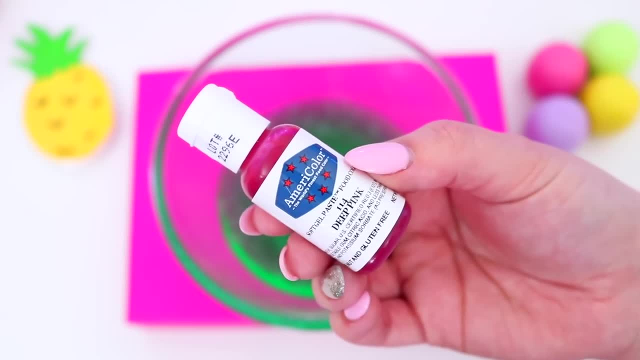 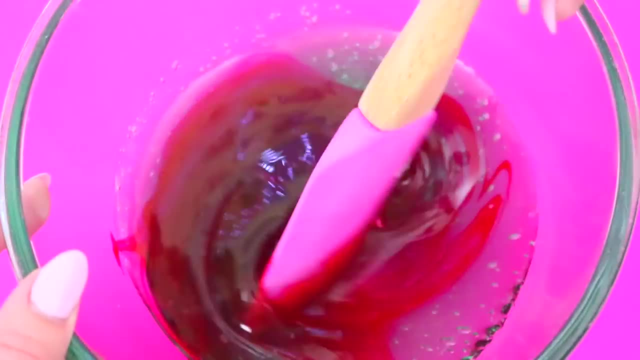 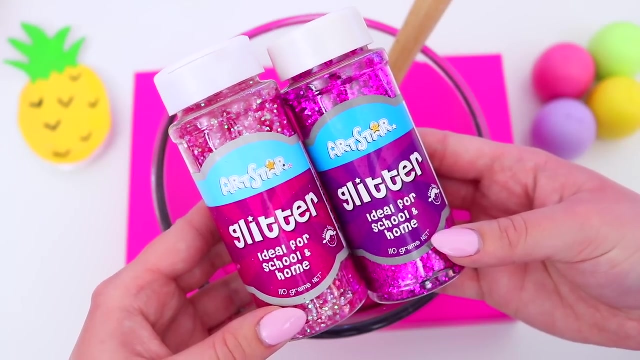 And then, if you want, you can make your glitter slime a really fun colour, and here I'm colouring mine pink and then just mixing in the food dye To finish off, I'm going to add this pink glitter slime, and it's just super easy. 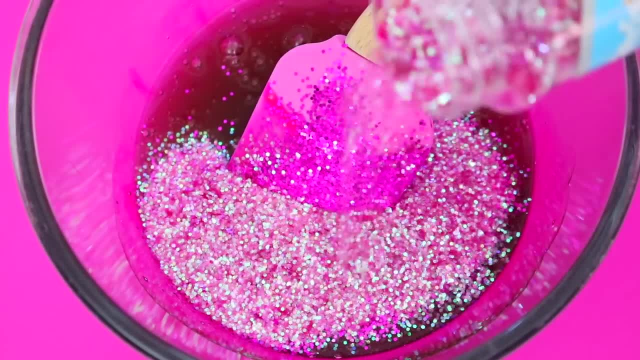 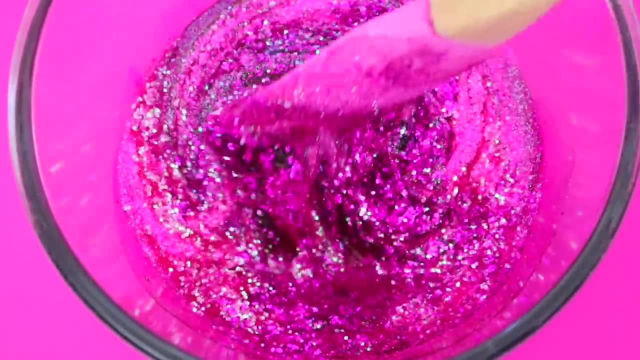 Next, for the fun part, you're going to need a bunch of glitter. so I just grabbed all the pink glitter that I had and started adding it to the bowl, and I love this part so much because it's just is so sparkly and magical. 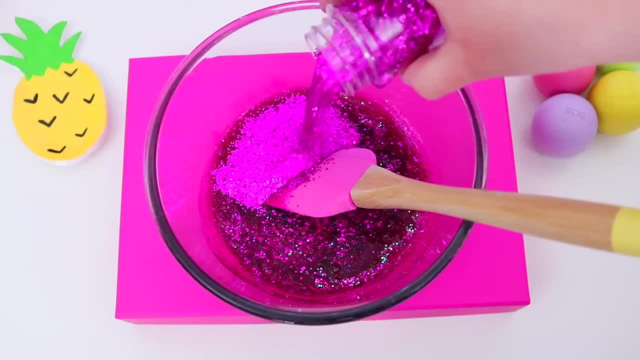 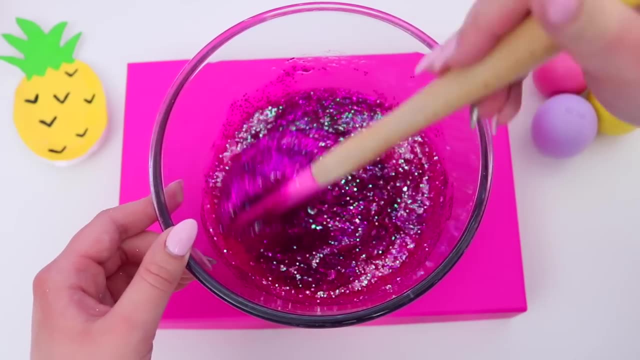 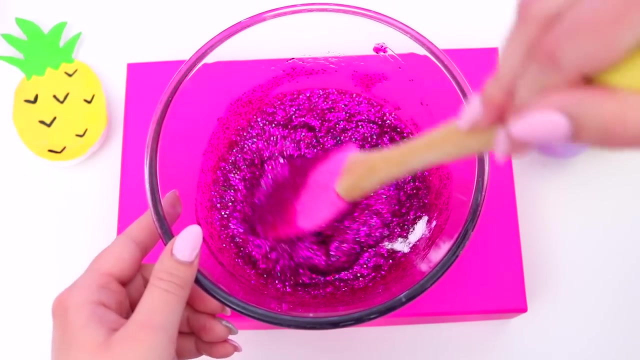 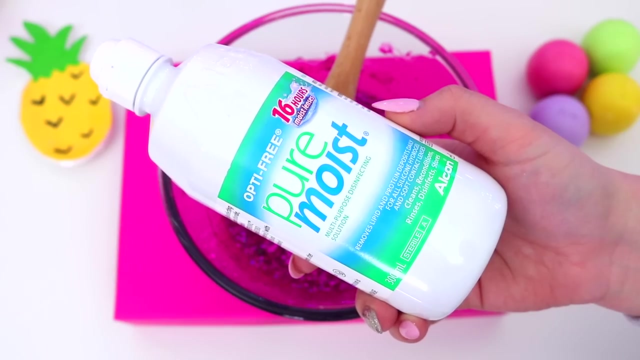 And then, once you've added all your glitter, you can just start to mix it into the face mask. my opinion: you can never have too much glitter. Then take just under a teaspoon of baking soda and add this to our glitter mixture and mix this in Now to activate our slime. we 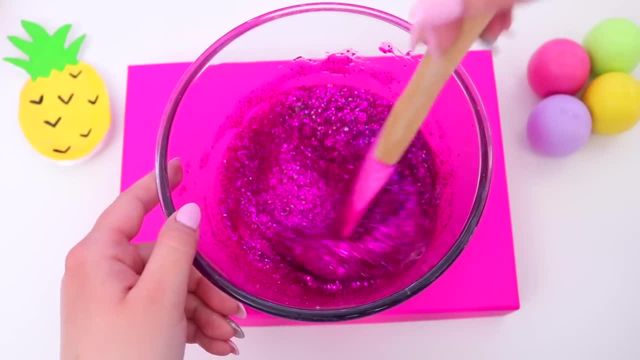 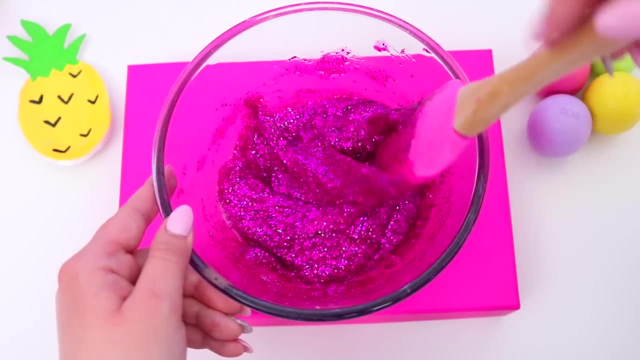 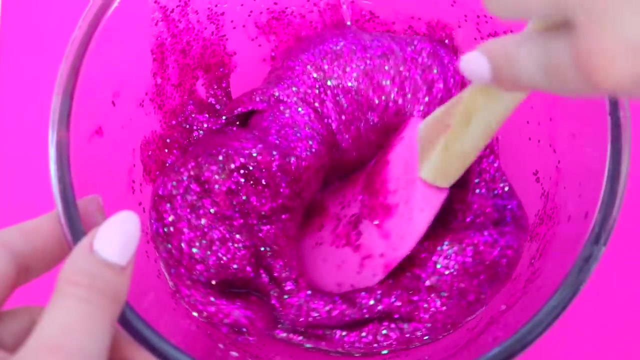 are going to be using contact solution. so just add a little bit of this at a time and mix it in, and then your slime will start to come together. So just keep adding contact solution until your slime is no longer sticking to the sides of the bowl, and then you can. 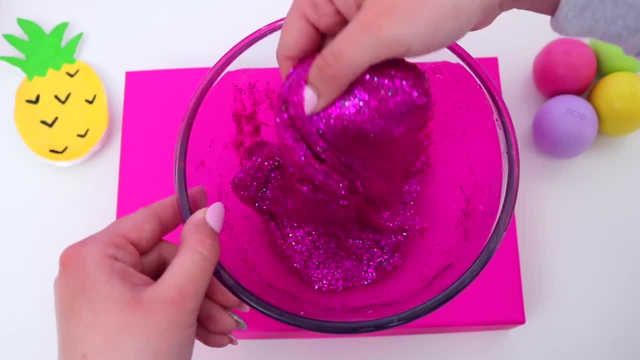 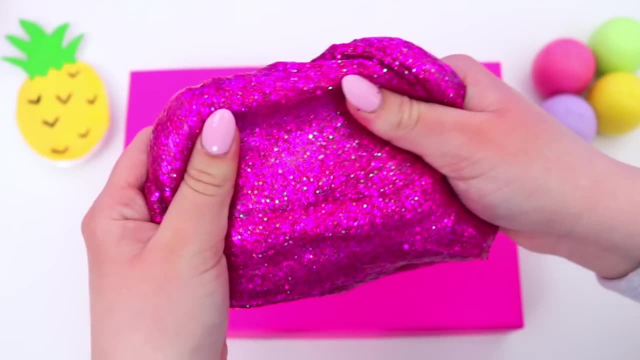 just go ahead and take it out of the bowl and start working it with your hands, and it should form the perfect slime. I love how sparkly this slime is and it's so pretty. I'm going to take a little bit of this and mix it in, and then we are going to be adding. 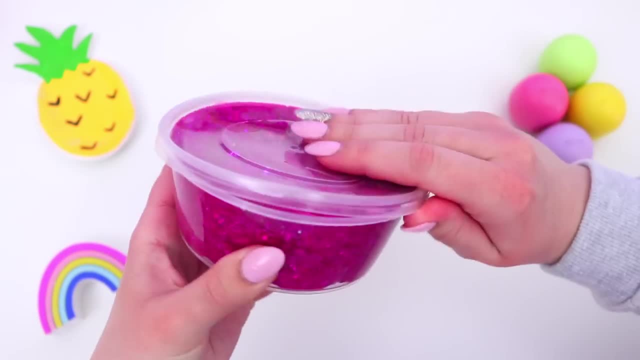 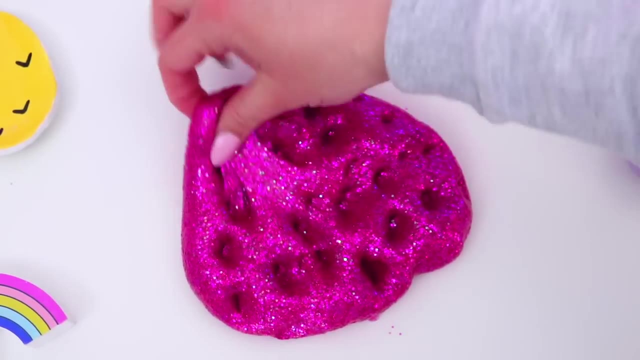 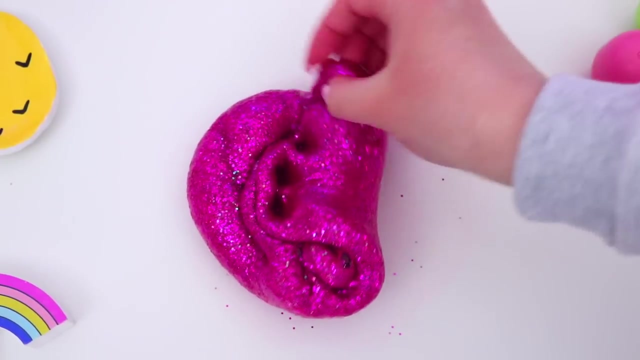 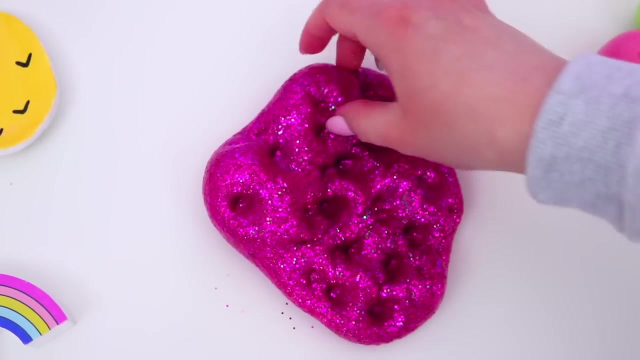 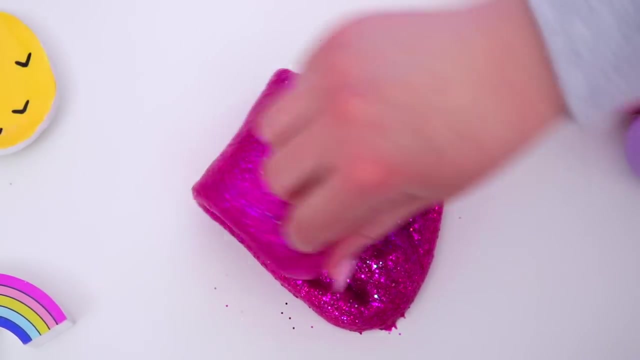 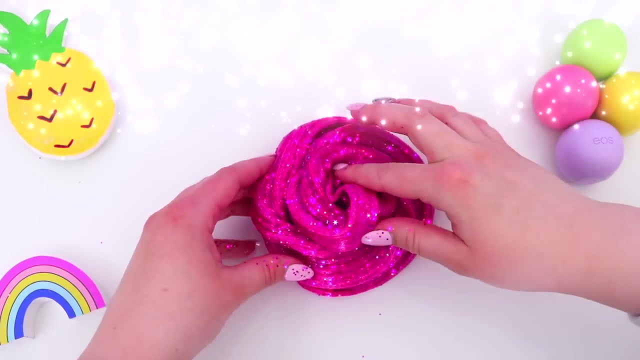 a little bit of the water to give the slime some texture. I can't believe this slime is made with no glue, because it totally feels like a slime made with glue and it's so easy to make and it's so pretty and sparkly and I'm just so. 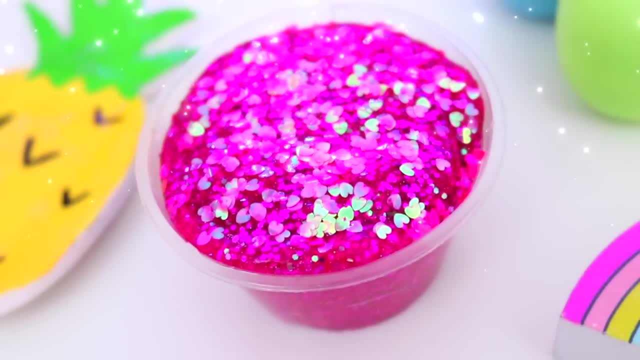 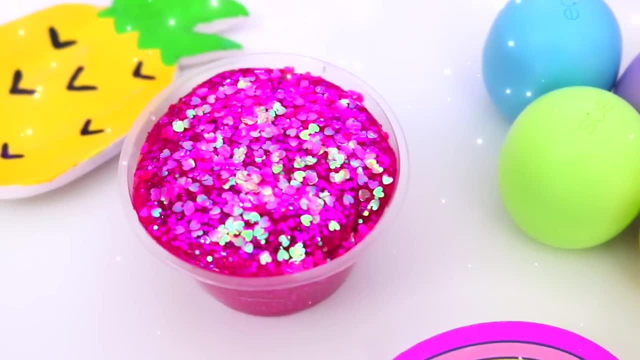 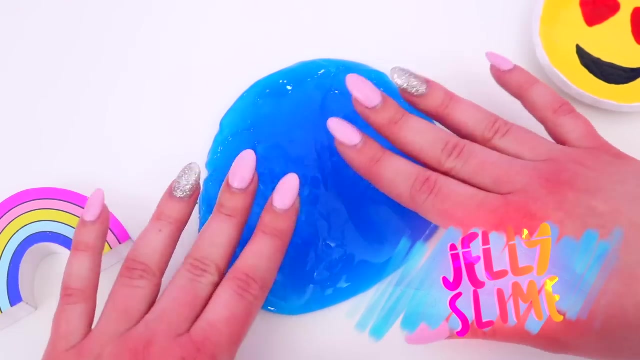 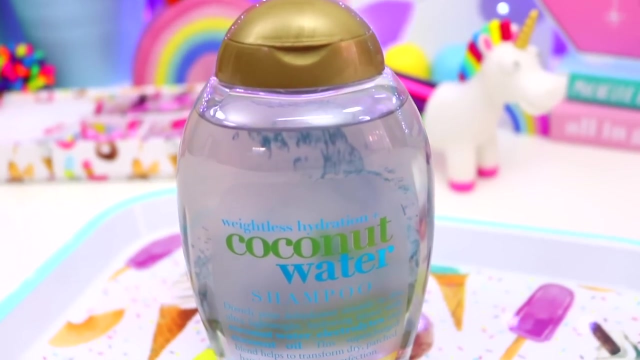 obsessed with it. Next, we have this jelly slime, and this isn't like a traditional slime texture. it's more, like I said, a jelly texture, but it's just so much fun to make and you can make it with ingredients that you can find at home, so I wanted to include it. 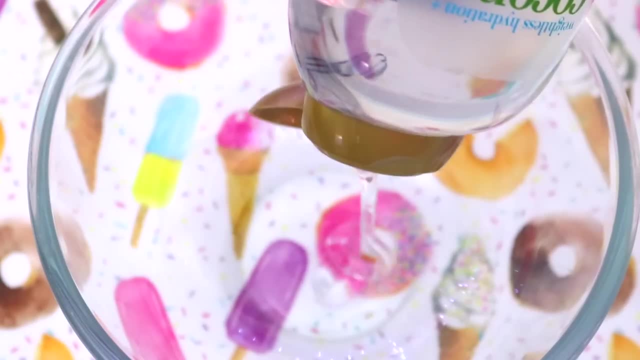 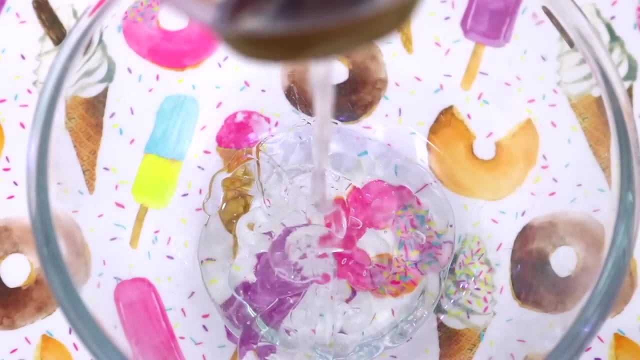 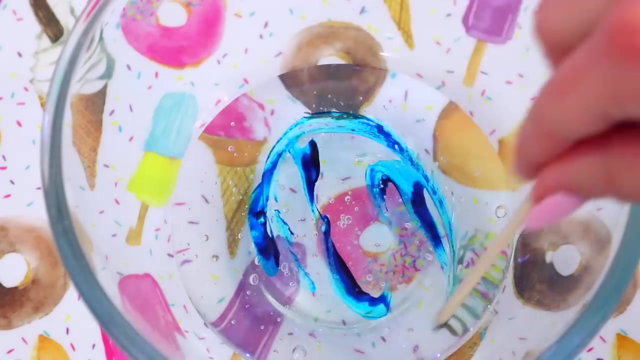 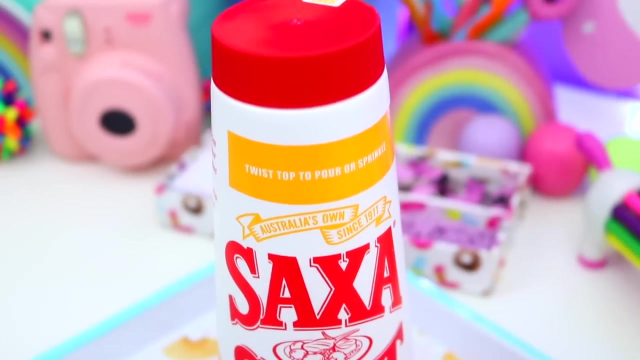 So, first, taking some shampoo, add this to a bowl. Then next I decided to colour this jelly slime blue, Because I love the way blue looks in clear slime. So I just added some blue food colouring and mixed this into the shampoo. Then you are going to need some salt, so I just went to the cupboard and found some salt. 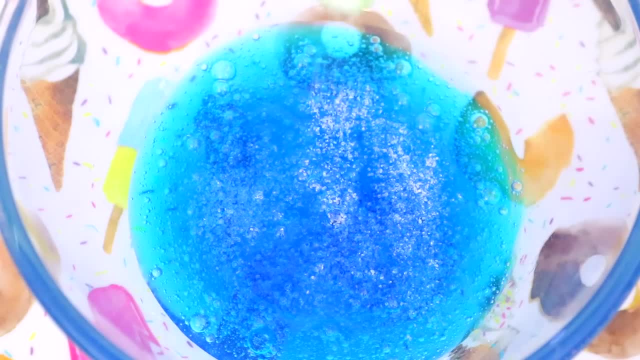 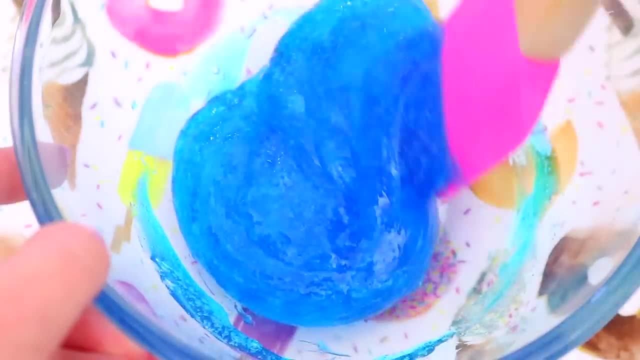 but you only need a super tiny amount of this and just sprinkle it on top of the shampoo and then start mixing it in, and you'll see that the texture of the shampoo will start to change. It becomes a little bit thicker and a little bit like actual slime. 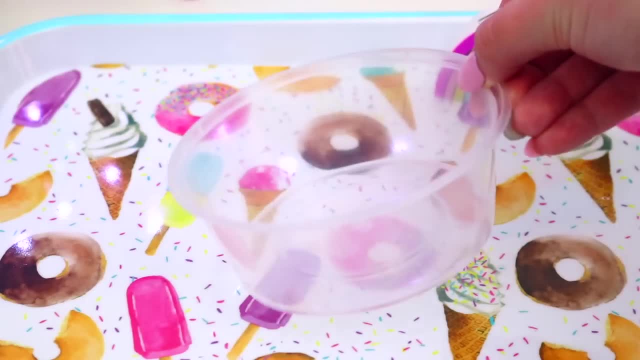 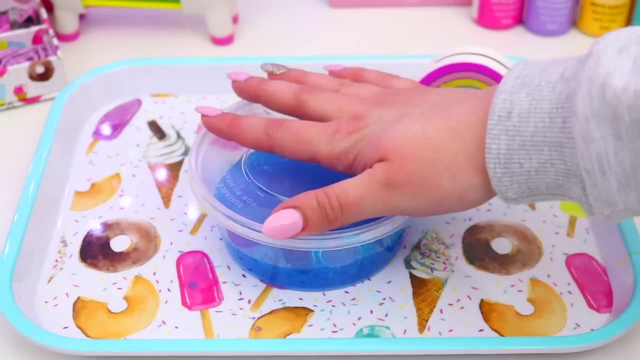 So then you just want to mix it in. Next, you just want to take a container and then, taking your shampoo mixture, place this inside of the container and then you just want to pop a lid on this and then pop it in the fridge for it to refrigerate for a bit and to cool down. 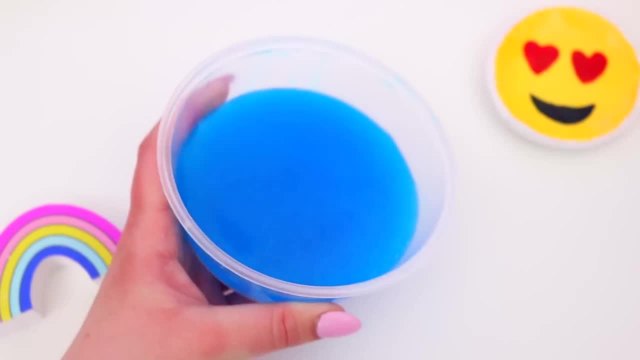 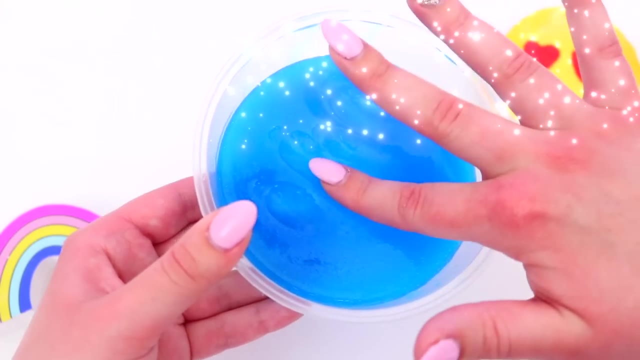 So, because it has been in the fridge, it has slightly solidified, so now you can like touch it and press it and it won't stick to your fingers. And, like I said, this isn't a traditional slime recipe, but it was just so much fun to make.